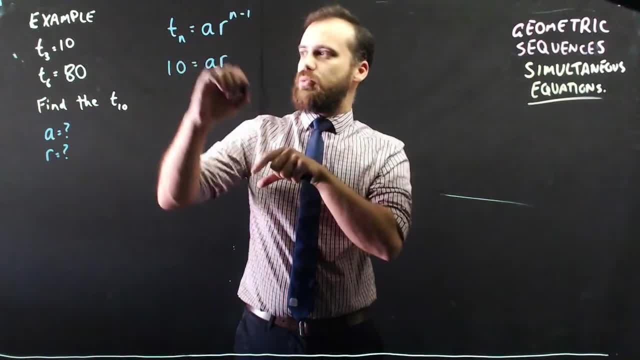 that if it's term 3, then it's going to be n minus 1, 2.. So 10 equals a r squared, and we know that term n equals a times r to the n minus 1.. So we know that term 3 is equal to 10. 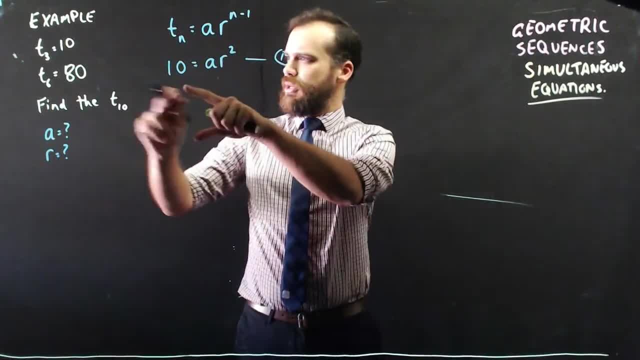 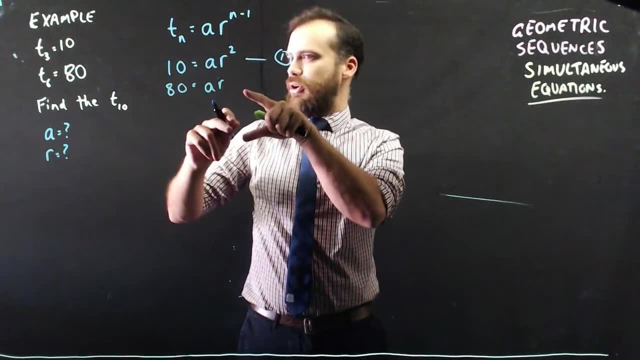 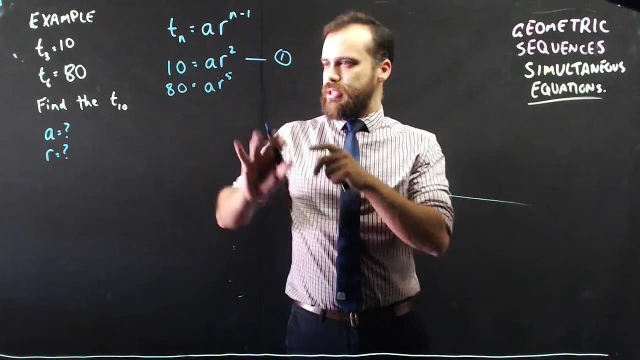 that's equation 1, and equation 2 is term 6 is 80 and that's going to be a r to the power of. if it's term 6, then it's got to be to the power of 5.. Now all we need to do is be able to solve. 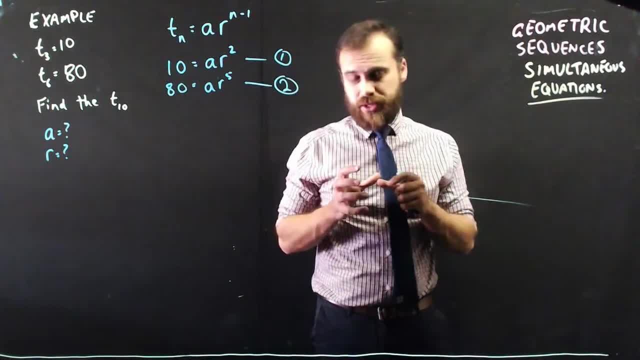 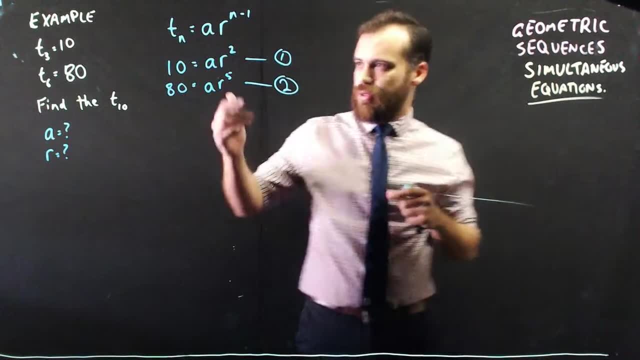 these simultaneously. Now there is a special way to do this that you've never seen before. You might remember doing elimination, simultaneous equations using elimination. The way that it works is: you're going to do a simultaneous equation and you're going to do a. 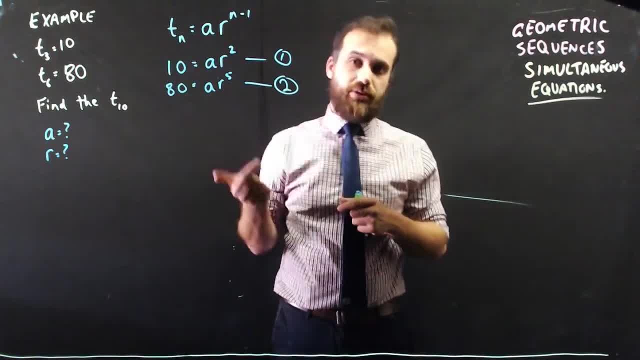 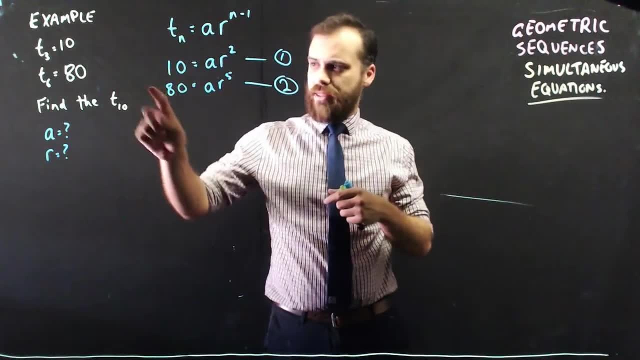 simultaneous equation. So what that works is: you take an equation and you subtract one equation from the other equation. Now, if you subtract one equation from the other, nothing's going to happen here, so that's not useful. You can also add them. if you add them also, nothing's going to happen. 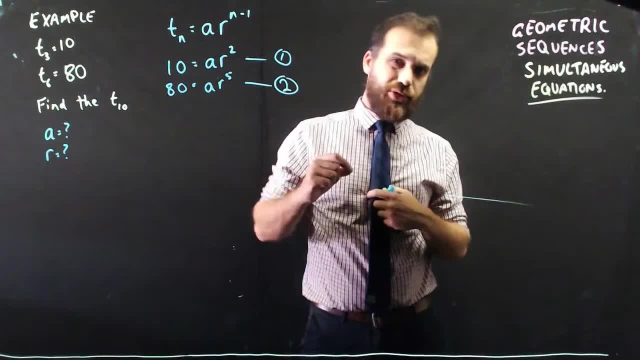 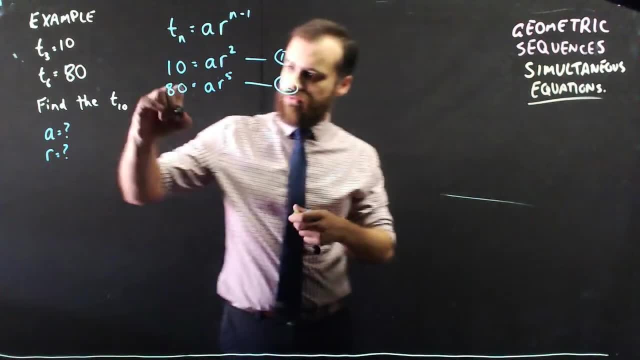 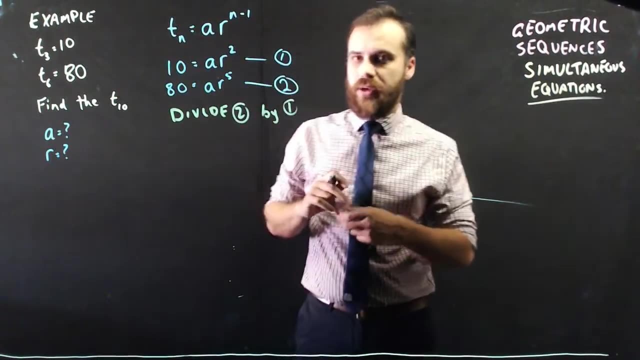 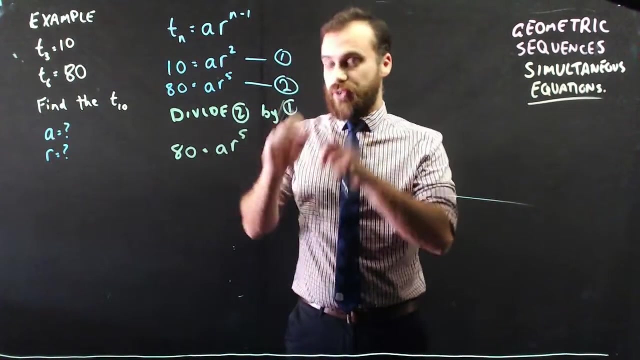 here, so that's not useful. but you can also multiply and divide them, which we've never done before, but you can do it. So if I write: divide equation 2 by equation 1, what that ends up looking like is: equation 2: 80 equals ar5 divided by equation 1. 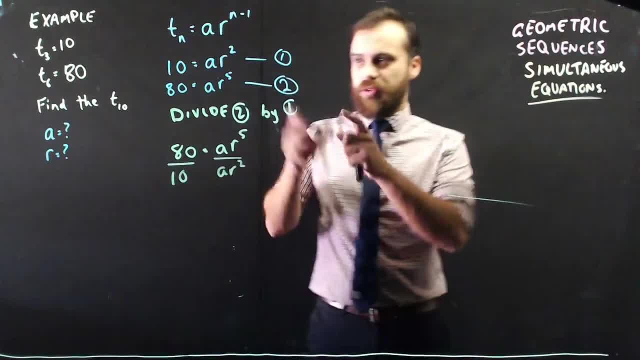 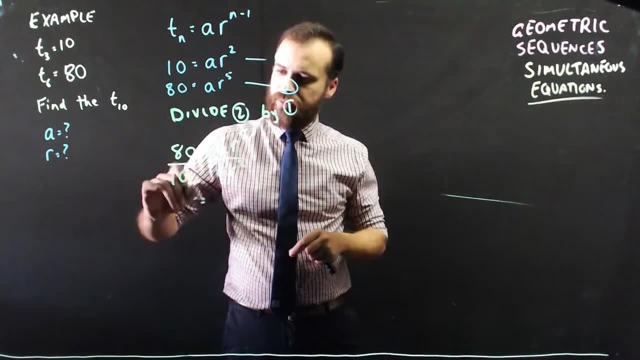 ar2.. Now you need to be really careful with this. it only really works with this kind of kind of format, and you'll see what happens. 80 divided by 10 is just plain old 8.. a divided by a: the a's will cancel each other out. 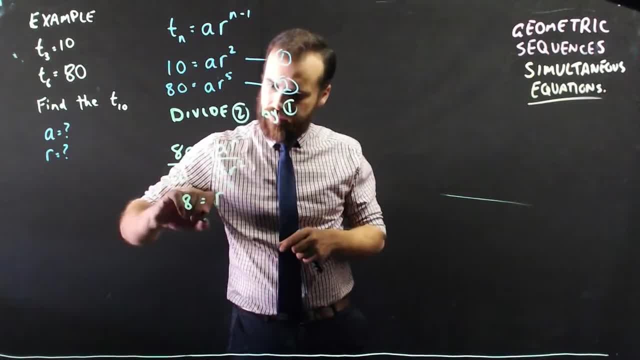 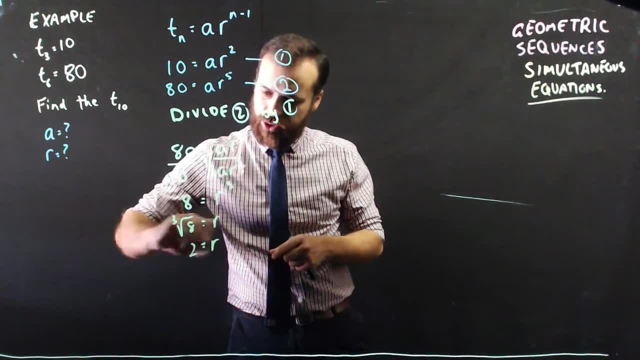 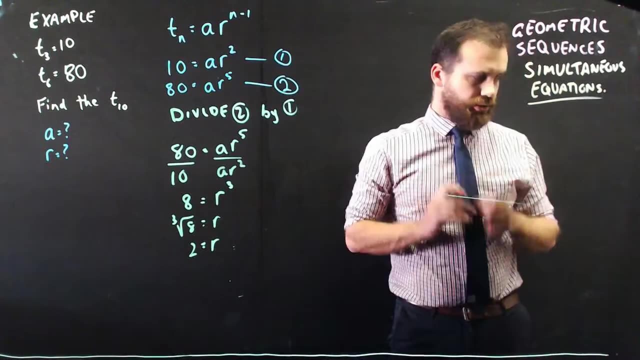 r5 divided by r2 will be r3, and then we end up with a cube root 8, so r is equal to 2.. Okay, that's our way to do it. You've never seen anything like that before. Just to show you there is a way to do it that you do know of, that you have done in the past. 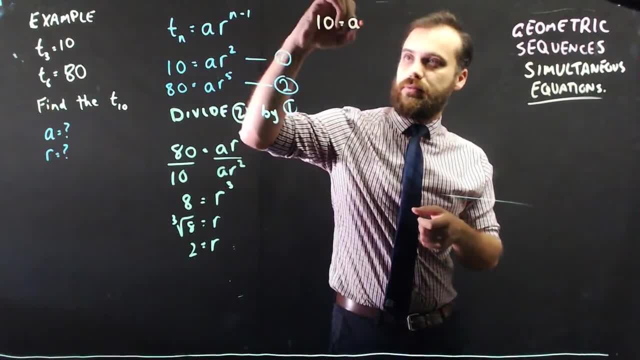 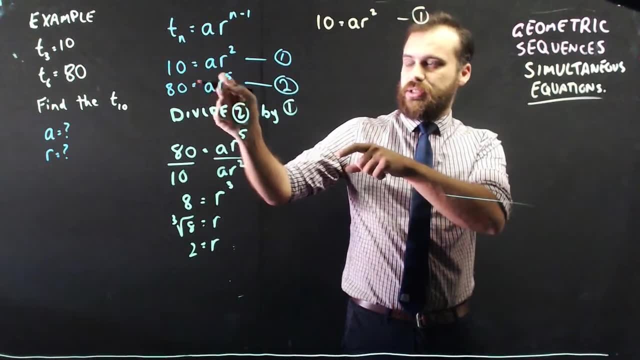 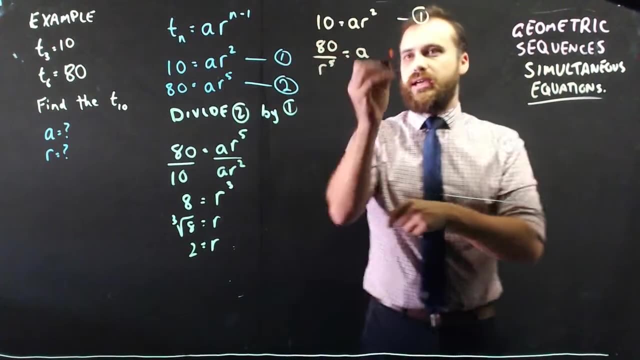 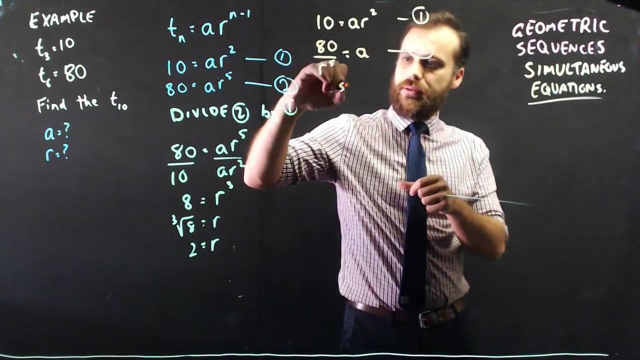 I can say that 10 equals ar squared, that's equation one, and I could rearrange equation two So that's equation two. So that means that equation two would be 80 divided by r to the five equals a. So now that I have that, I can use substitution. I can sub two into one for a. 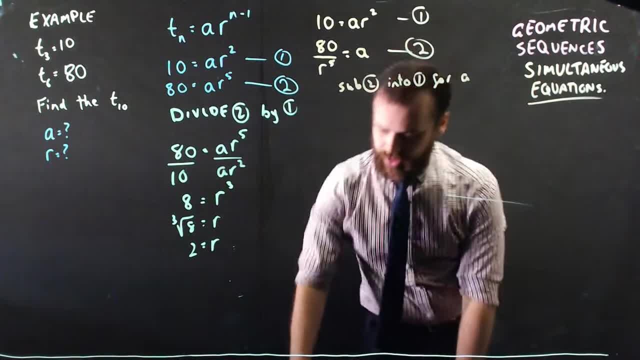 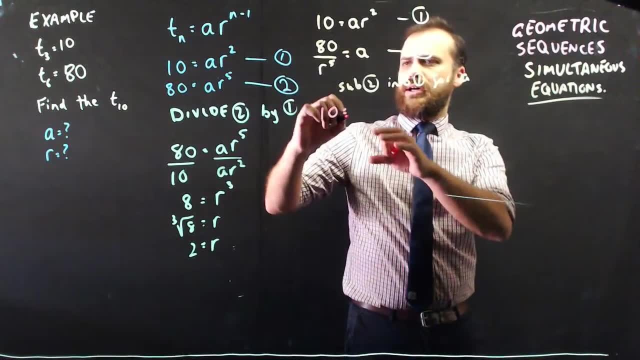 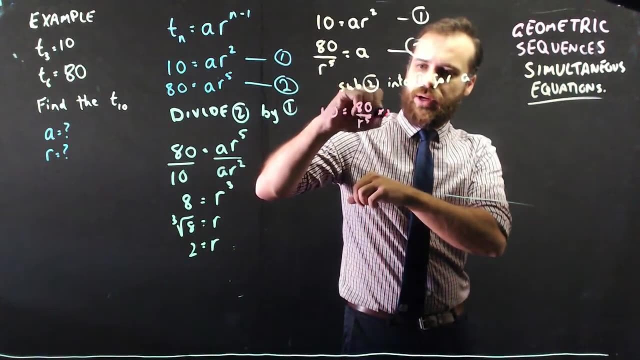 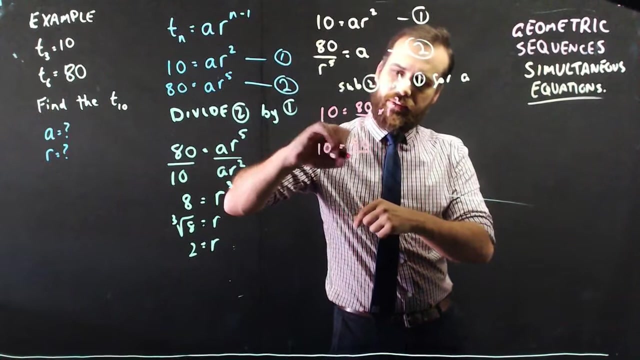 So it's going to be. let's use a different color here so you can see what's happening. I'm trying a different one: 10 equals. substituting that in, we get 80 over r to the five and then multiplied by r squared: Okay. so that's going to give me 10 equals 80 r3.. 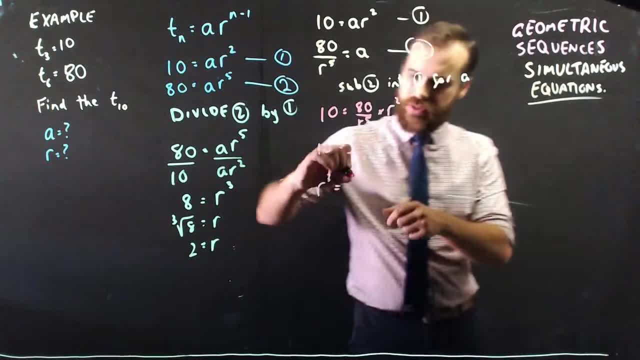 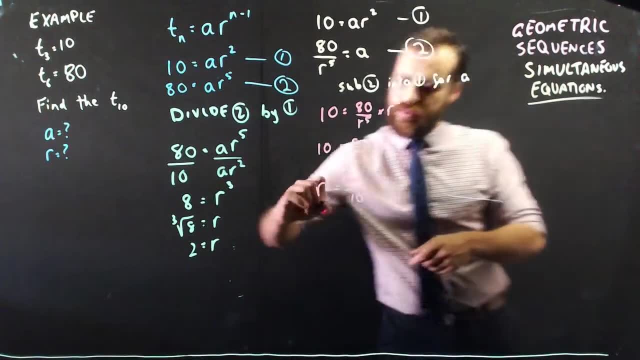 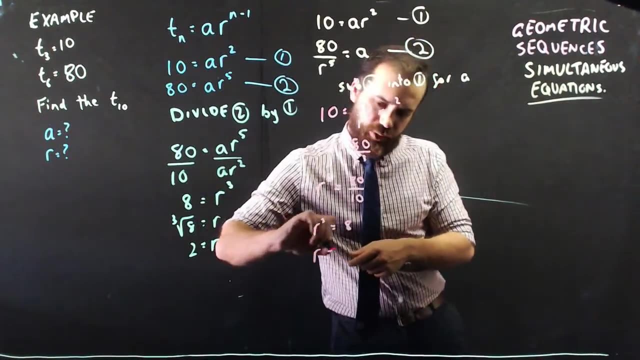 I can move r3 to the top using a cross multiplication. we end up with 80 over 10.. And you should see that r30 equals 80 over 10.. 10 out of the 3 equals 8, which means we're here. so r equals 2.. 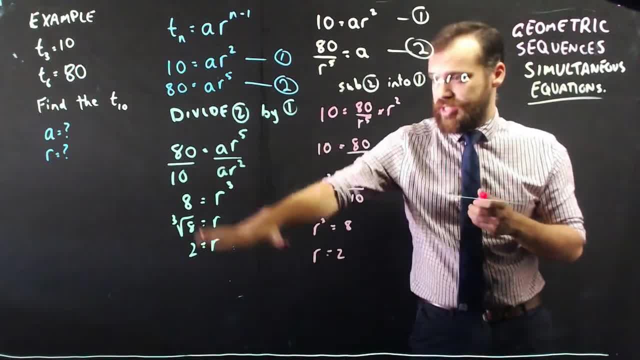 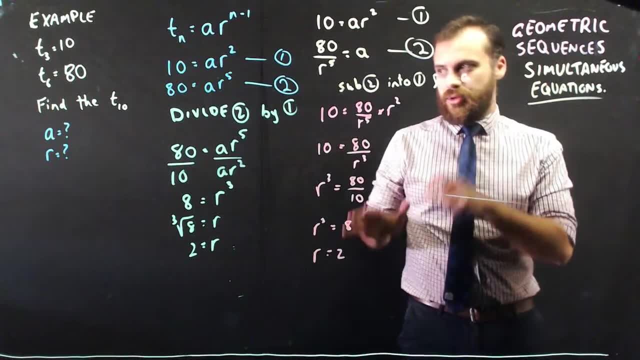 Okay. so it doesn't matter which way you do it. You can use that fancy dividing method or you can use this method, which you have seen before, But now we know that r equals 2. We need to know what a is now. 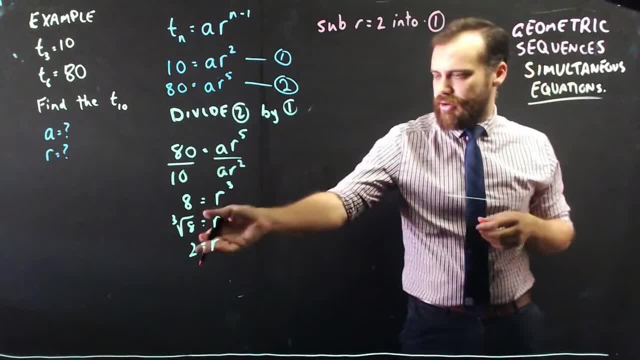 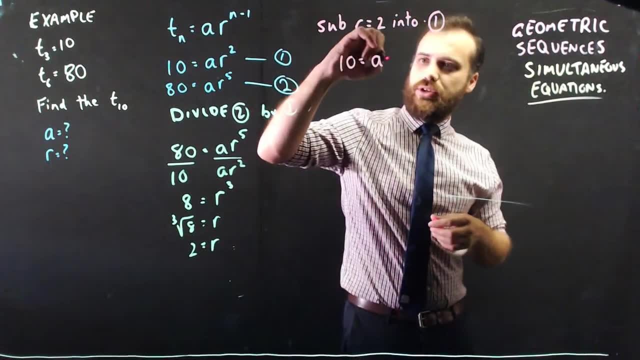 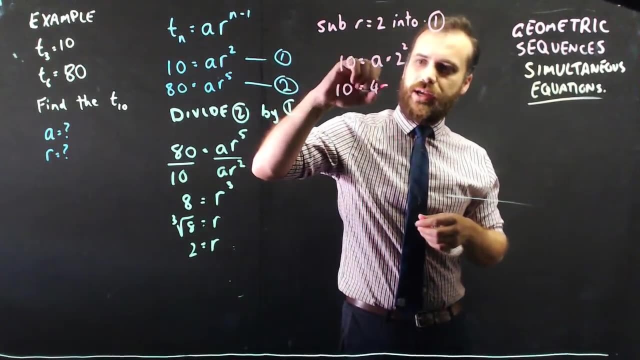 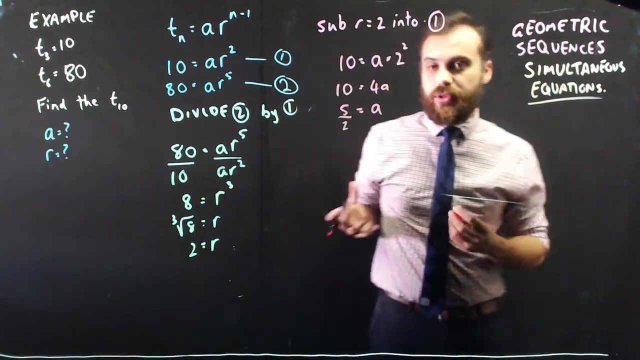 I'm going to just get rid of some of this. So now that I know r equals 2,, I can sub r equals 2 into equation 1.. So 10 equals a times 2 to the power of 2.. So 10 equals a times 4, or 4a, which means that a equals 10 on 4,, which is 5 on 2, or 2.5,. 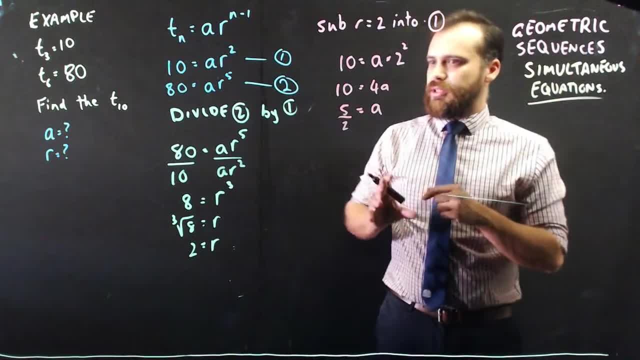 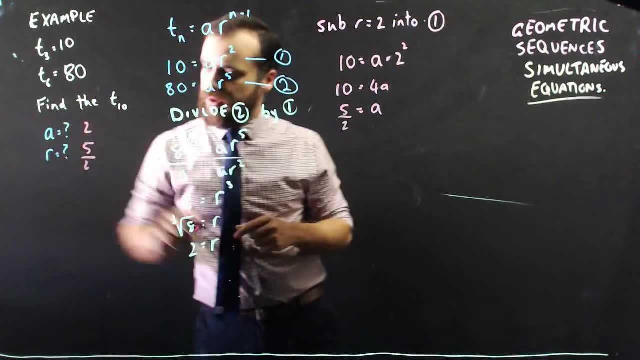 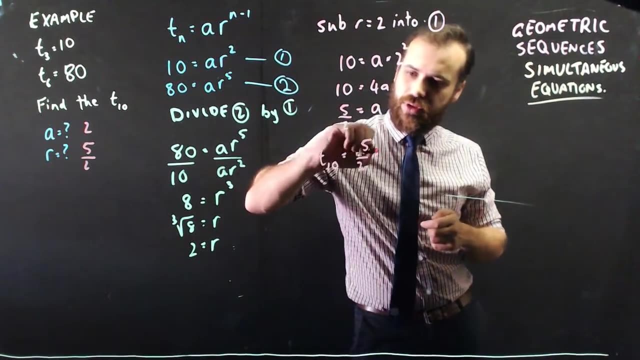 whatever you feel comfortable dealing with. Okay now, finally, that's the hard bit. Now that we know that a equals 2, and we know that r equals 5 on 2,, we can find out that r equals 2.. We can find the 10th term by saying: term 10 equals a 5 on 2, times 2 to the power of 9..